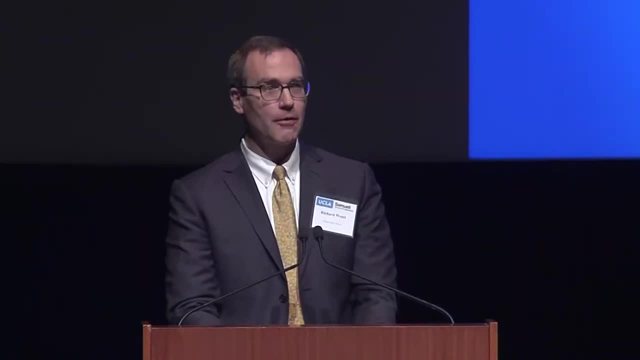 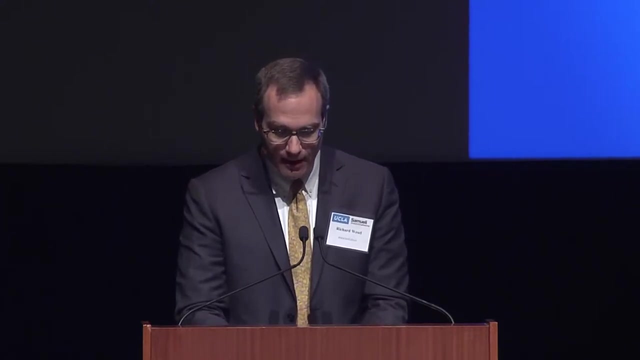 As part of Professor Lee's exciting research profile, he develops techniques to use endogenous stem cells to repair damaged arteries. When most people think about biology at the cellular level, they think about chemistry, But one of the unique approaches of Professor Lee's work is to focus on the physics of action at the cellular level to better understand how cells function. 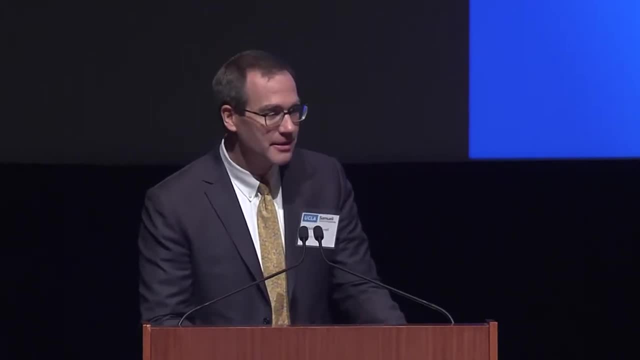 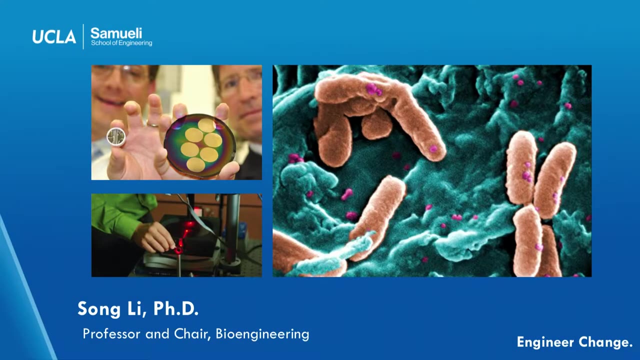 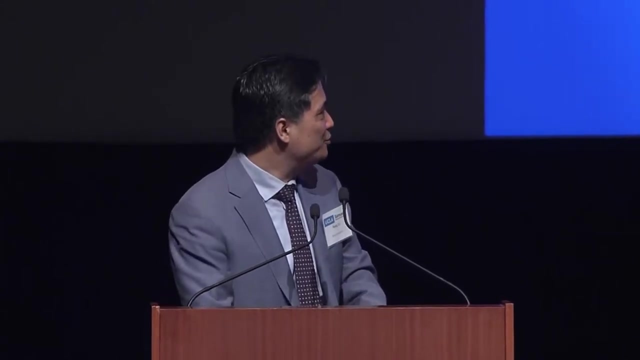 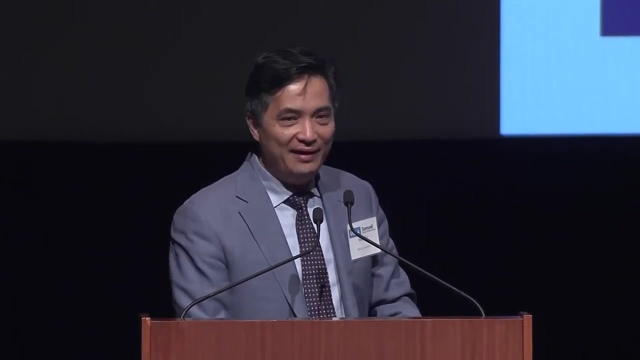 And to explain to you better how the biology of cells function And to explain to you better how the bioengineering department functions. here is Professor Lee. Good morning everyone. Bioengineering is actually a relatively new department in engineering school and it has grown very fast in the past two decades. 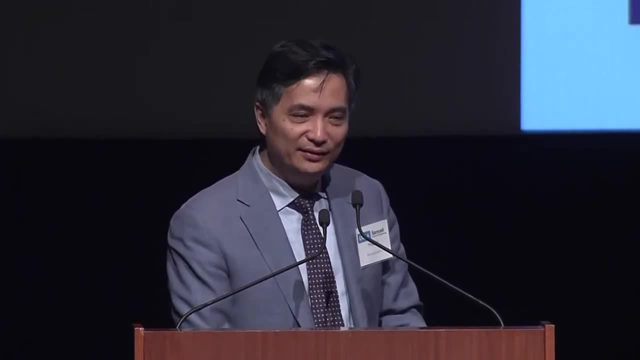 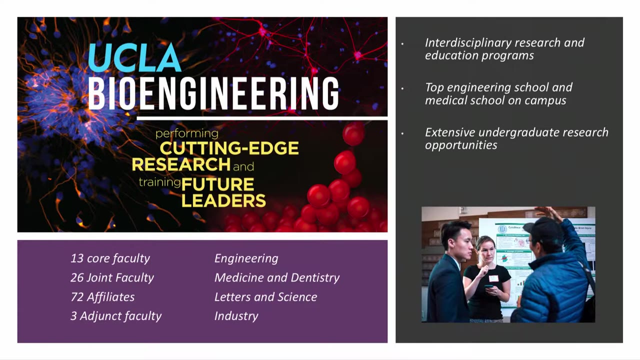 Bioengineering as a field actually is quite interdisciplinary And you could see, actually in our faculty we have many faculty in engineering, core faculty and joint faculty, but many affiliated faculty actually in medical school, in other colleges, for example letters in science. 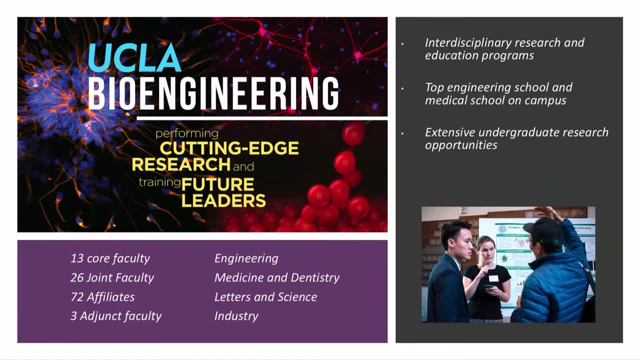 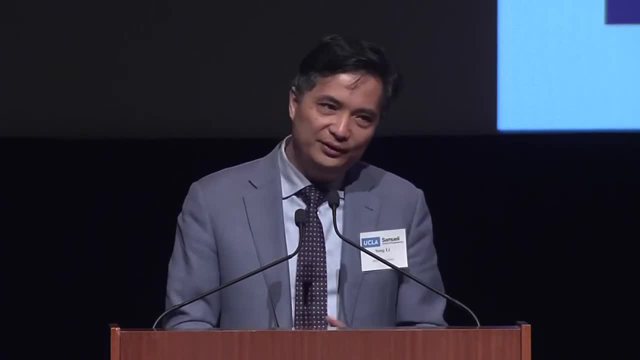 And we also have adjunct faculty teaching biotechnology classes from industry. So at UCLA we have a very unique situation. Both top engineering and medical schools are online. We are on the same campus, It's very close by to each other and that gives us a lot of opportunity for bioengineering research and education. And, for example, our undergrads for research experience. over 90% of the undergrads have done at least one year of research and more than 60% of them have done at least two years of research, And this is the highest percentage in all UC bioengineering program and compared to all other schools it's also very high. 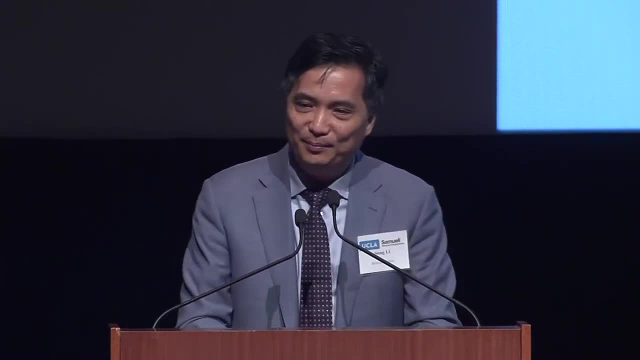 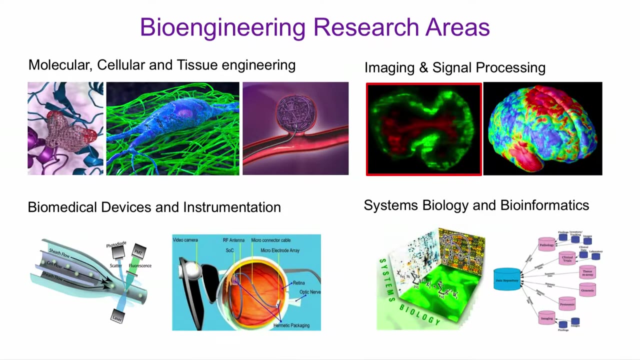 So here I want to show you some examples of what we do in the department. Bioengineering is a very broad field and here we focus on four areas. One is molecular, cellular and tissue engineering. You can see here on the top left. 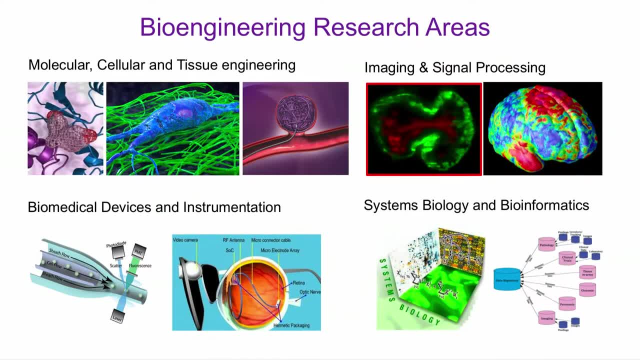 At the molecular level, we engineer micro and nanoparticles and use that for drug delivery or use that for imaging process. And at the cellular level, we work on stem cells And we use the stem cells And we use the stem cells for the regeneration of tissues in organs. 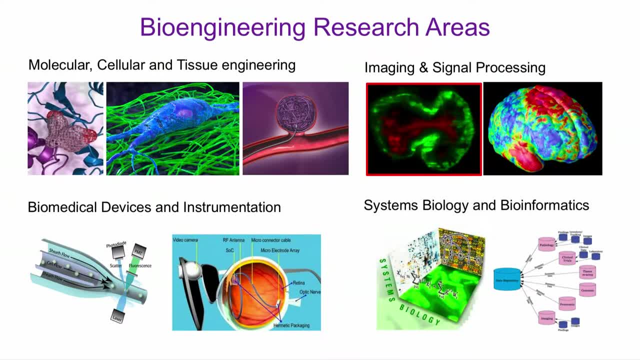 And the second area is biomedical devices and instrumentation. This includes both micro devices for point of care, application for diagnosis, And also some example here you can see this is actually a pair of high-tech glasses our faculty developed. In this case it's to help blind people to see again.